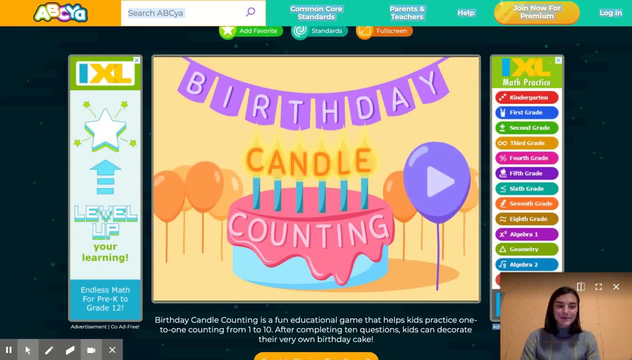 Good morning everyone. My name is Ansley Brunk and I am so excited to be here to interview for the second round for a teaching position at the AC Charter School. So today I'm going to use a tool from the internet and a website called ABCYAH to introduce a counting lesson. This lesson is: 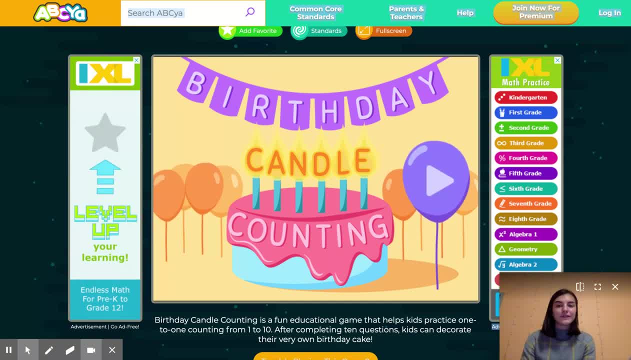 really appropriate for kindergartners or first graders and it's a great starting point or an introduction for a counting lesson. ABCYAH- a little bit of background on that. there's a wide variety of subjects and from kindergarten math and reading all the way up to like algebra. 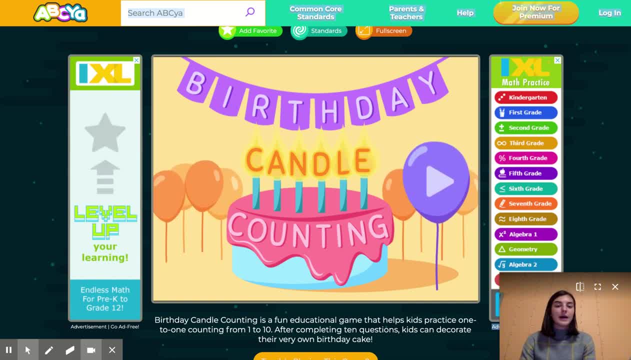 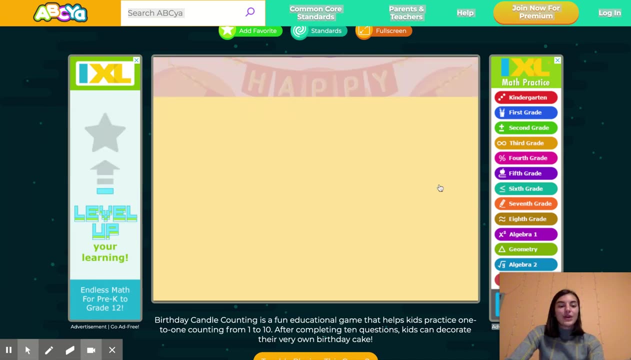 2 and geometry. So it's a great learning tool for students of all ages. So let's get started on our counting lesson. So the game I would like to use to introduce our counting lesson is birthday candle counting. So when you start with birthday candle counting, click on the candles to count. it reads the: 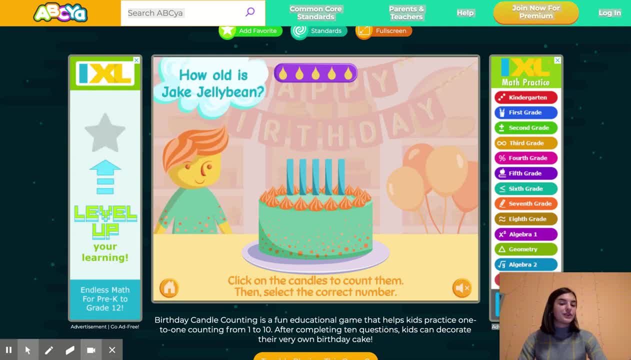 direction. so it says: click on the candles, then select the correct number. So this game not only gives you options to count, but it also gives you a question that students have to answer to go with the counting method. So to answer um, you have to go through and you have to click on each of the candles. 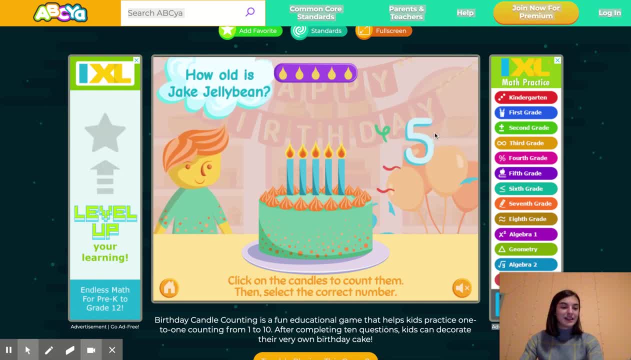 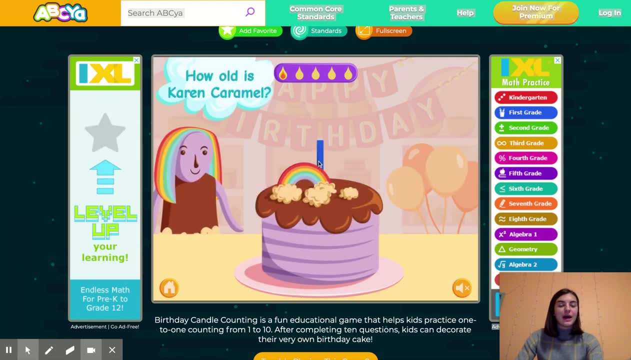 and then balloons pop up with answer choices and then they click the correct, correct answer choice that goes with it. Uh, a vital point to this game is that once you click on the candle, it says the word out loud, which is so good, especially when introducing a counting. 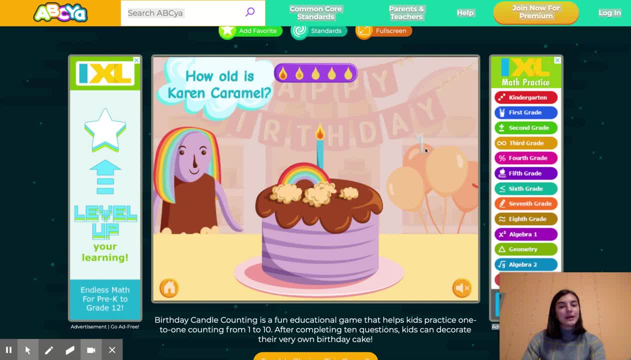 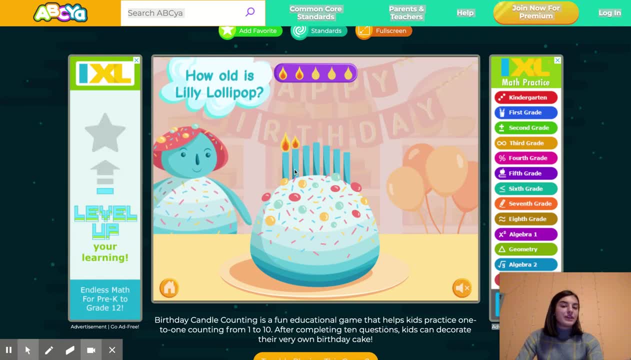 lesson for students. So they click on the correct number, they answer the question correctly and then they continue to move on to each question: How old One, Two, Two for independent work as well, because as a starter you can have it say and then your kids repeat: 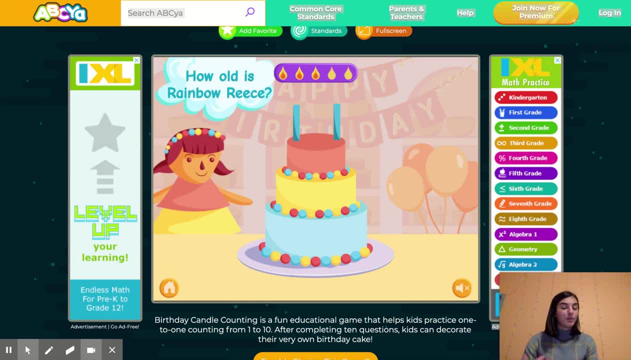 the number or how's their profession and counting. they can count that. So it's a good thing for them to work on individually or on their as a group so you can put it up on the smart board and have kids interact and click on the candles themselves and really interact with counting and hearing.